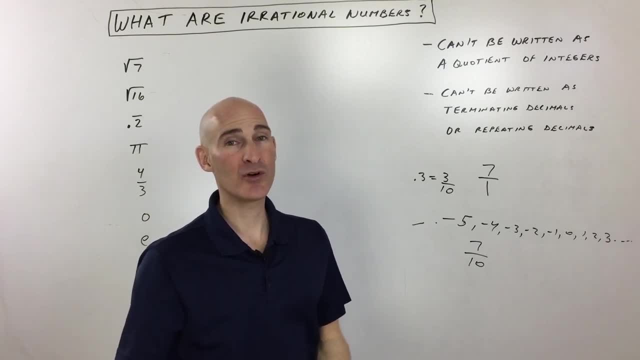 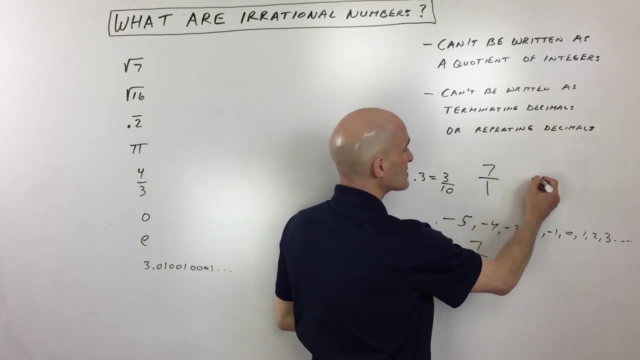 you can see, we're back to an integer divided by an integer. That's a rational number, not an irrational number. And then also it cannot be a repeating decimal. Now, a repeating decimal would be something like this: 0.2 repeating. So this is actually 0.222, dot. 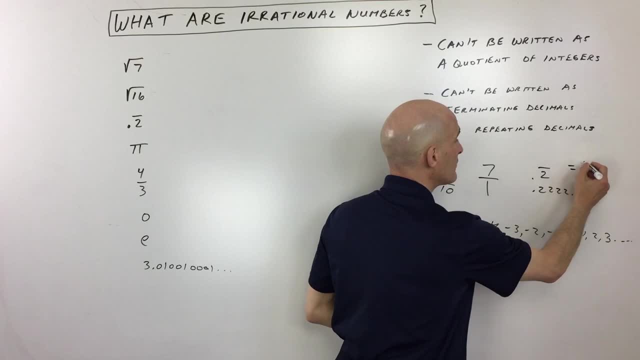 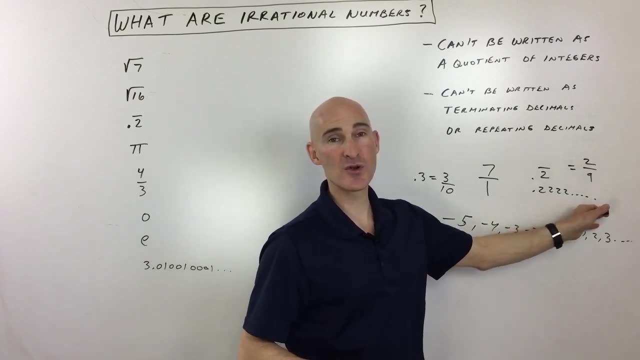 dot dot right, And that can actually be written as a ratio of an integer divided by an integer. It's 2 divided by 9.. And you can check that by dividing that on your calculator and you'll see that you get 0.2 repeating So with irrational numbers. let's take a look. 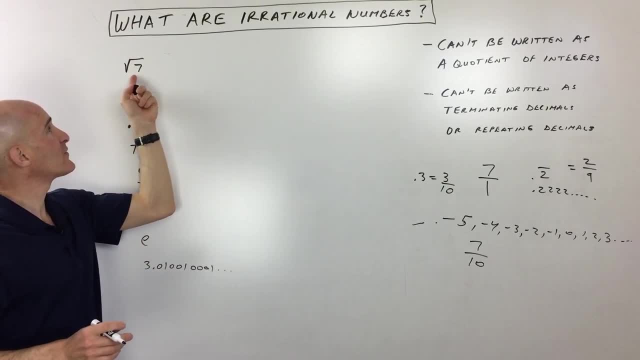 at some examples, see if we can classify these. So say, for example, the square root of 7.. Okay, square root of 7, if we do that on our calculator, you're going to see that it's a square root of 7.. So, if we do that on our calculator, you're going to see that it's a. 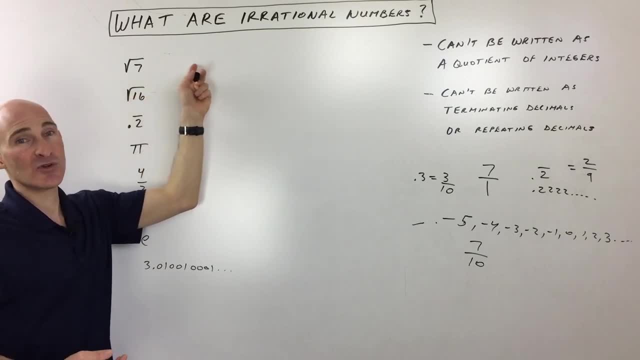 non-terminating, non-repeating decimal, So this is actually an irrational number. Okay, square root of 16,, on the other hand, can be simplified to 4, because 4 squared is 16, and 4 can be written as a ratio of an integer divided by an integer. So this: 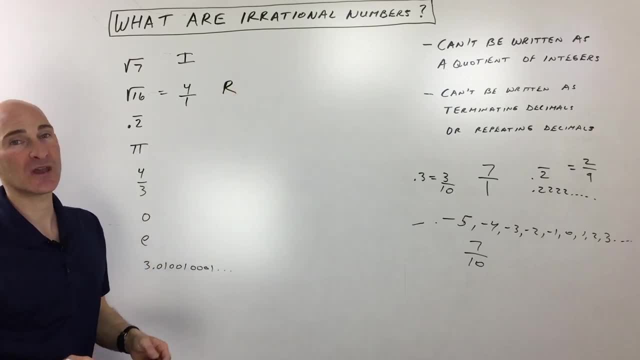 is actually a rational number. I'll just put R for rational. Okay, 0.2 repeating. that's the one that we did over here earlier. That's actually a ratio of an integer divided by an integer. It's a repeating decimal, so that's actually going to be rational. 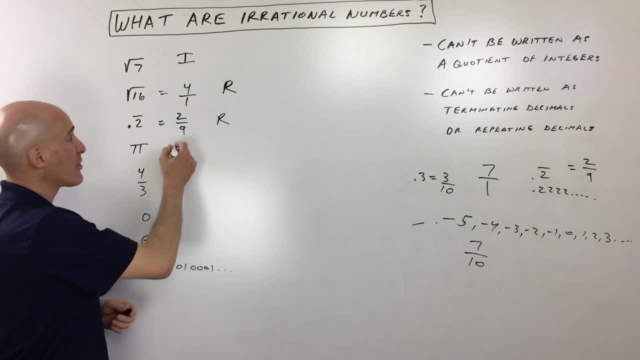 Pi, on the other hand, is approximately right: 3.14159 dot, dot, dot. Now it doesn't repeat and it doesn't terminate or stop, And so this cannot be written as a ratio of an integer divided by an integer. so this is an irrational number. Okay, 4 thirds 4. 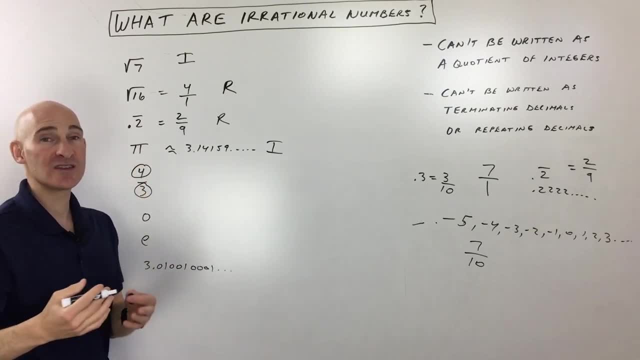 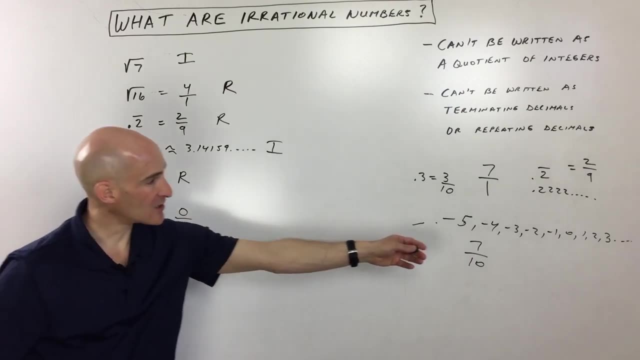 thirds, you can see it's already a ratio of an integer divided by an integer. This is a rational number. Okay, R for rational Zero can be written as zero divided by one. So zero is an integer, as we talked about over here. One is also an integer, so it's a ratio. 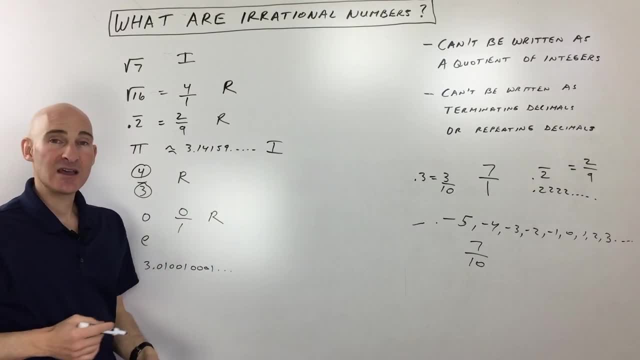 of integers. That's a rational number. E is approximately. it's a number like pi, where it's 2.71, dot dot, dot. It doesn't repeat, it doesn't terminate, so that's considered an irrational number. And then this last one here, 3.01001001,. this one tricks students.